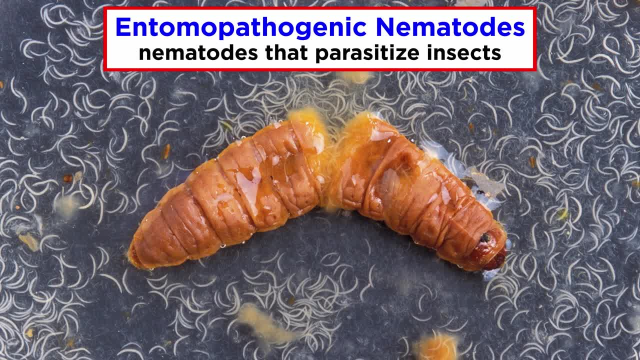 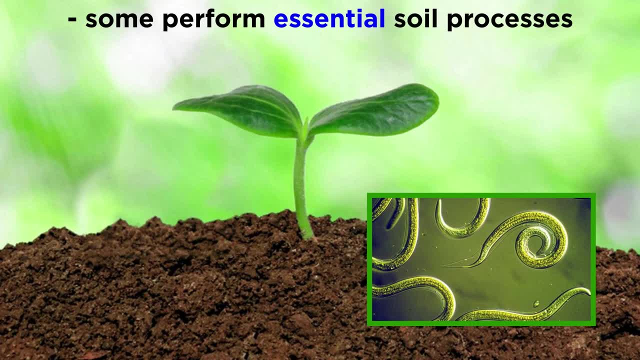 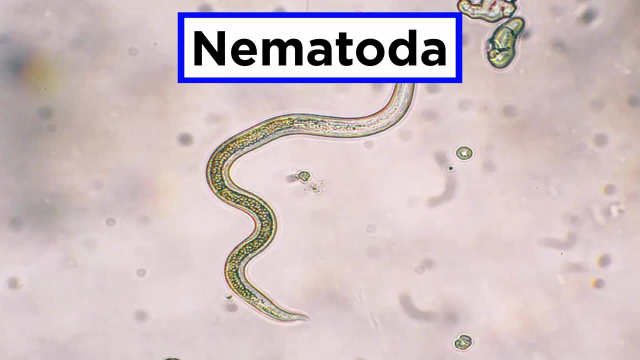 to seriously reduce populations of insect pests and have even been applied as a type of biological pesticide, while others perform essential soil processes and still others cause massive damage to economically important crops. In order to better explore this diverse phylum, we will go over form and function and how they can be used to bone Shoreworm, which is the main source of food. 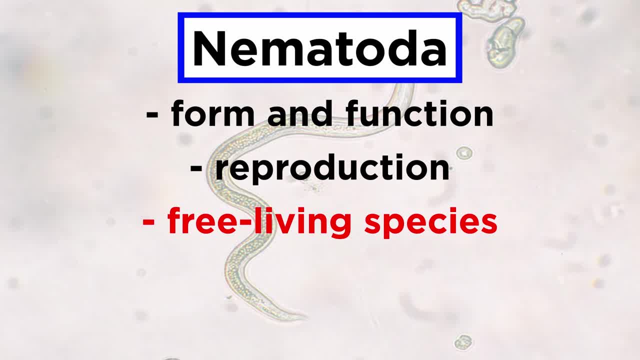 and other controlled, unhygienic or highly restrictive environmental and even toxicIES. About 25% of the most described nematodes are found to have been found in the soil and about 50% of them are reproduction free-living species nematodes in agriculture. and, finally, the importance of 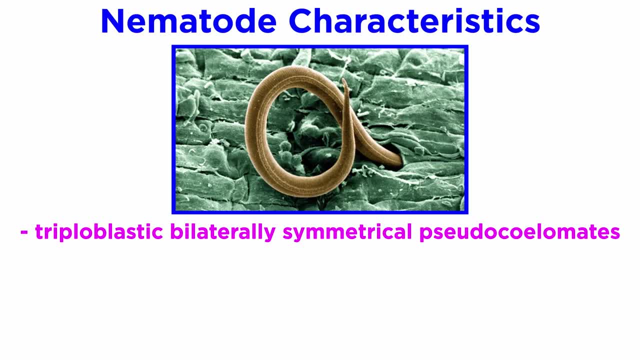 C elegans. All nematodes are triploblastic, bilaterally symmetrical pseudocelomates. They are cylindrical in shape, flexible, with unique body wall. muscles, lack cilia and demonstrate utile, also known as cell constancy. Utelic organisms have a fixed 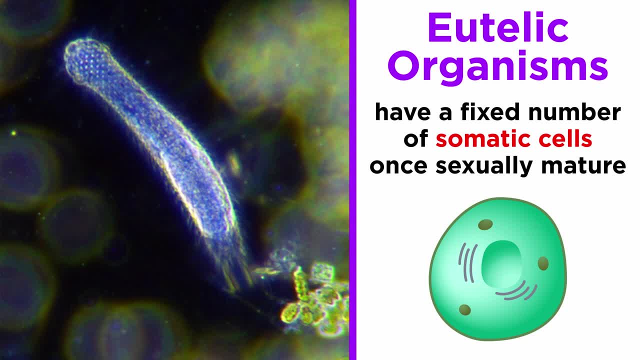 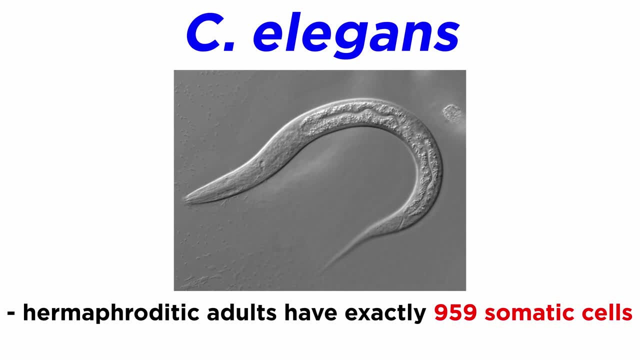 number of somatic or non-reproductive cells when they reach sexual maturity. For example, hermaphroditic adults of the species C elegans will always have exactly 959 somatic cells, while males of the same species will always have 1031 somatic cells. Note that this only applies. 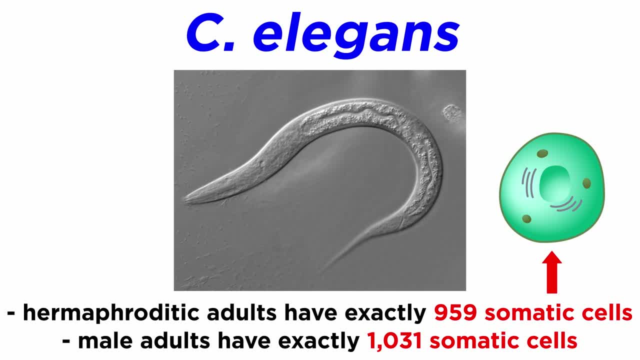 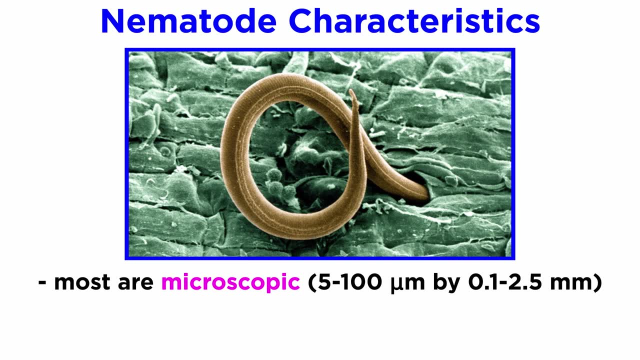 to somatic cells. The germ cells or sex cells may vary from individual to individual. Most nematodes are microscopic, Usually 5 to 100 microns thick and 0.1 to 2.5 millimeters long. However, some free-living 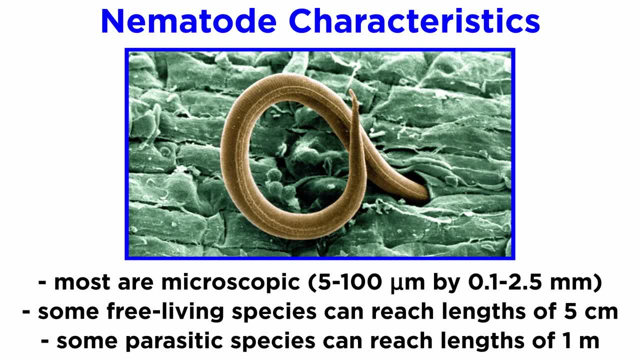 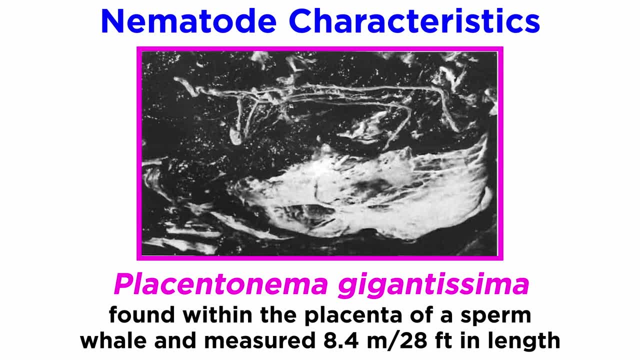 species can reach sizes up to 5 centimeters, and some parasitic species can reach lengths of 1 meter or more. In fact, in the 1950s, one species of giant nematode, Placentanema gigantissima, was recorded within the placenta of a sperm whale as being 8.4 meters or about. 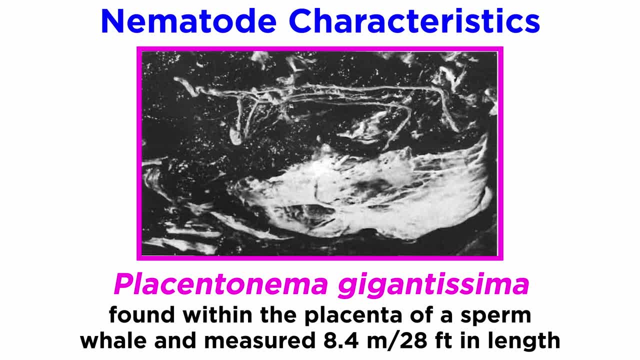 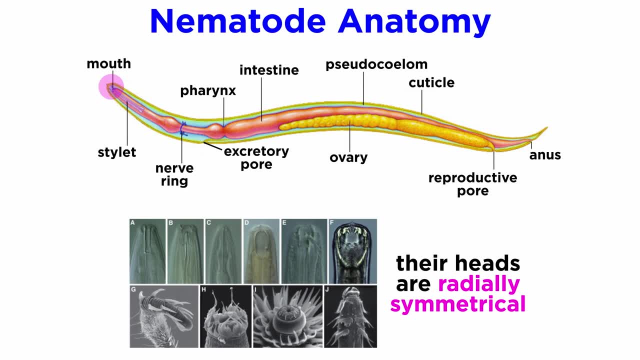 28 feet. Placentanema gigantissima is the largest nematode ever described, but such sizes are quite rare. Most nematodes have head regions that are distinctly radially symmetrical, in contrast with the rest of their bilaterally symmetrical body, and often come equipped. 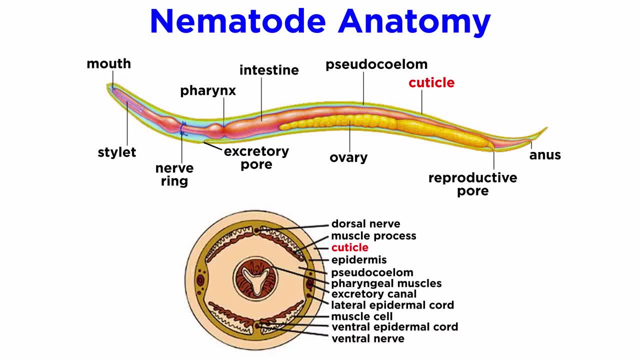 with three or six lips and a series of teeth. Their outermost layer is their characteristic protective cuticle, under which lies their thin skin-like epidermis. Underneath the epidermis lies their muscular skin-like epidermis. Underneath the epidermis lies their muscular. 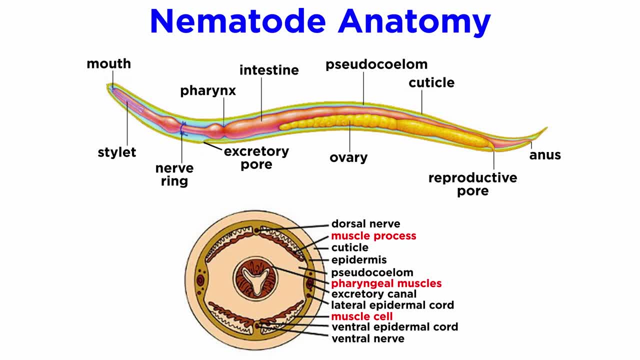 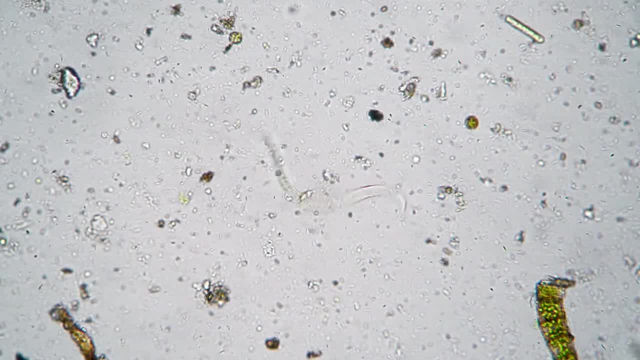 skin-like epidermis, The musculoskeletal or maxillofacial muscle system, which is comprised mainly of a layer of longitudinal muscle cells. These muscles work in conjunction with the cuticle and fluid-filled pseudoseal to constitute a hydrostatic skeleton. This skeleton provides 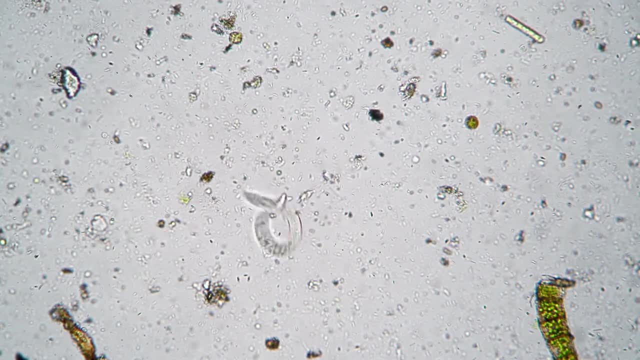 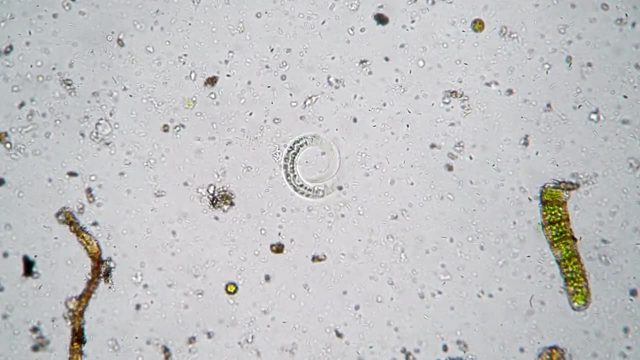 support for the roundworms by transmitting the force of muscular contraction to the enclosed non-compressible fluid, thus allowing the nematode to move. This hydrostatic skeleton is necessary for many aspects of nematodon. Thanks for watching life history. 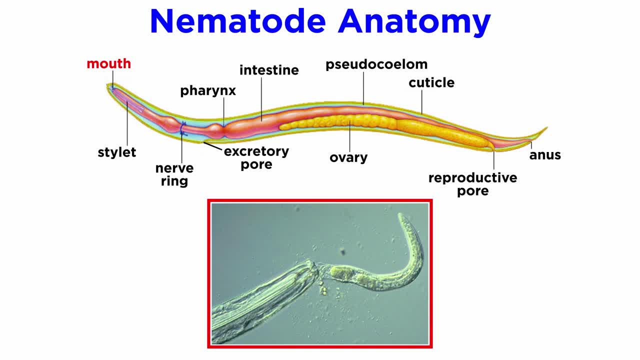 The digestive system, for example, begins with the oral cavity. Many nematodes have a sharp stylet that they can use to capture prey. Captured prey is moved into the muscular pharynx, where digestive glands produce enzymes that start to break it down. 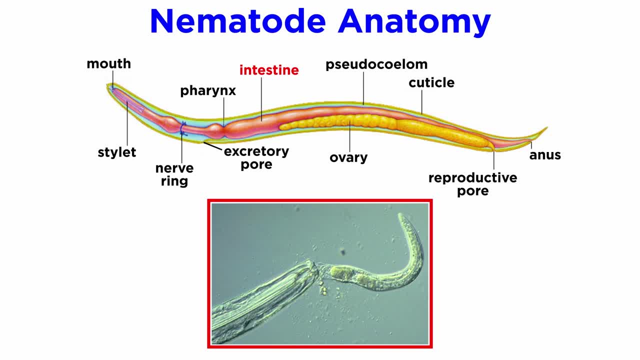 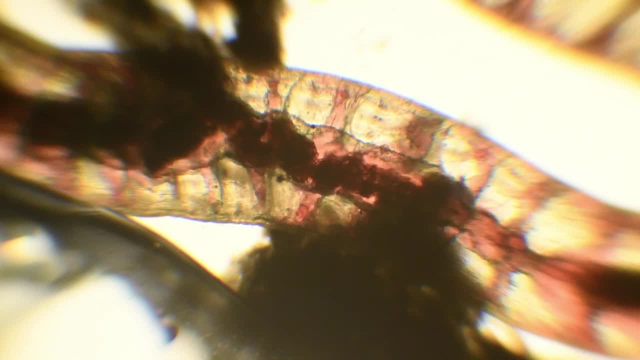 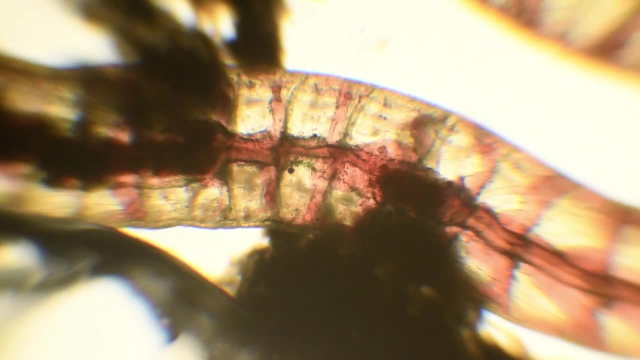 Nematodes have no stomach, and the pharynx instead connects to muscleless intestine that runs the length of the body and terminates at the rectum and anus. Since there are no muscles in the intestine, the food that moves through the digestive system does so by movements of the body mediated by the hydrostatic skeleton. 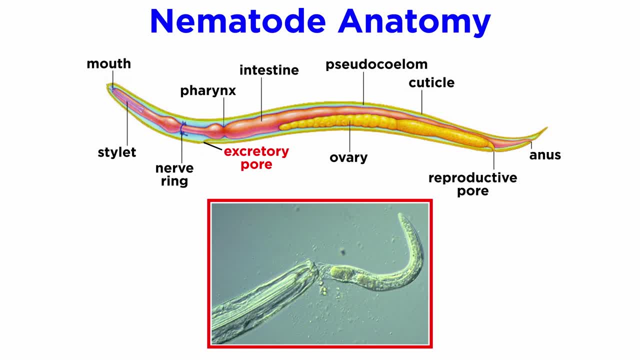 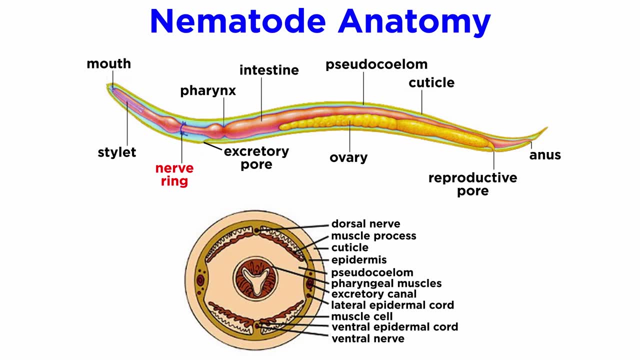 Nematodes excrete nitrogenous waste through their body walls and lack any excretory organs. Their nervous system is made of a dense circular nerve ring which surrounds the pharynx and acts as the brain. Several smaller nerve cords extend anteriorly towards the oral cavity and larger nerve. 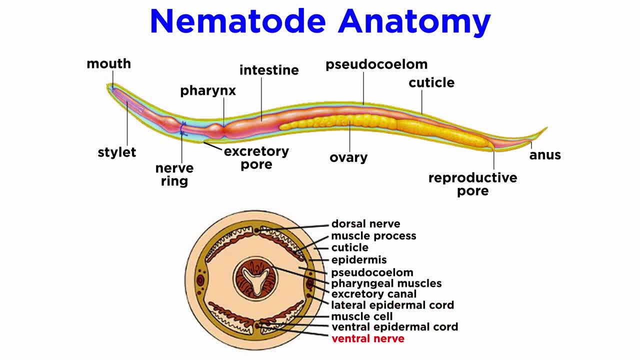 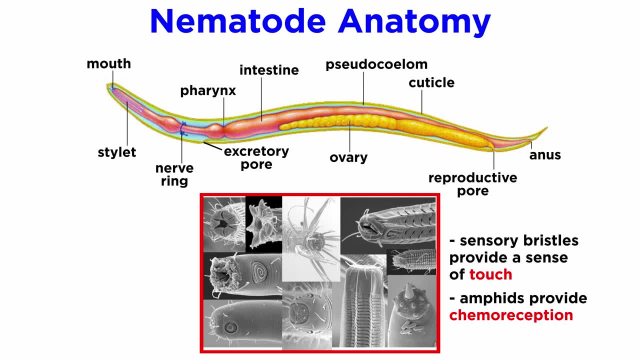 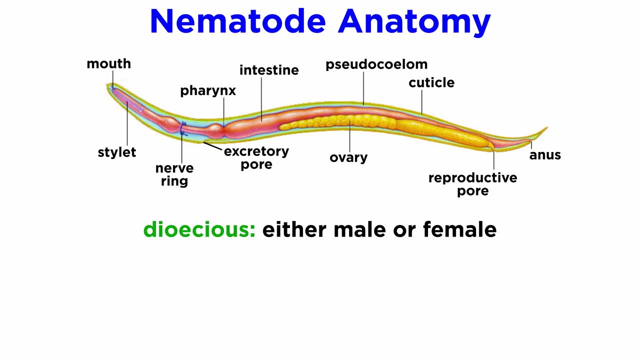 cords extend posteriorly. The largest of these is the ventral nerve cord. Nematodes are also covered in sensory bristles that provide a sense of touch and smaller organs known as amphids, which are responsible for chemoreception. Most species of nematodes are dioecious, meaning male or female, or androdioecious, where most. 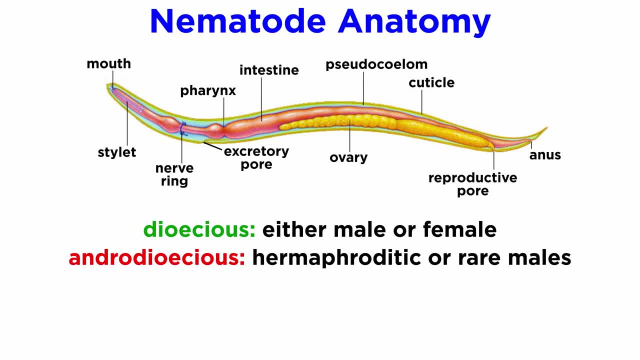 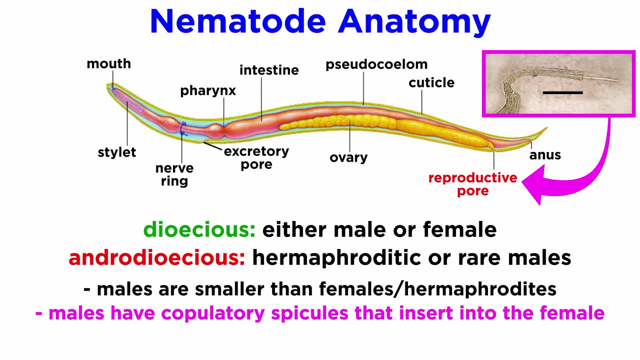 individuals are hermaphroditic, except for rare males that only display one sex. Males are often smaller than females and hermaphrodites and are equipped with a pair of copulatory spicules that are inserted into the genital pore of the female. 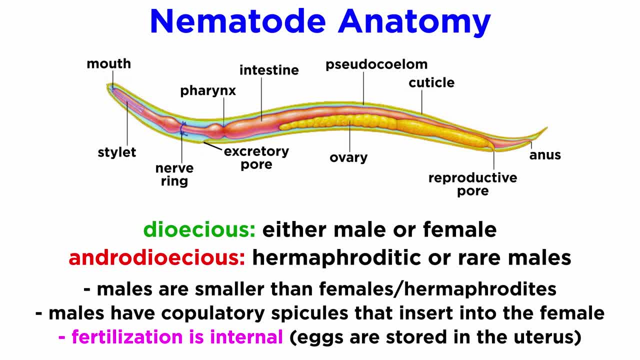 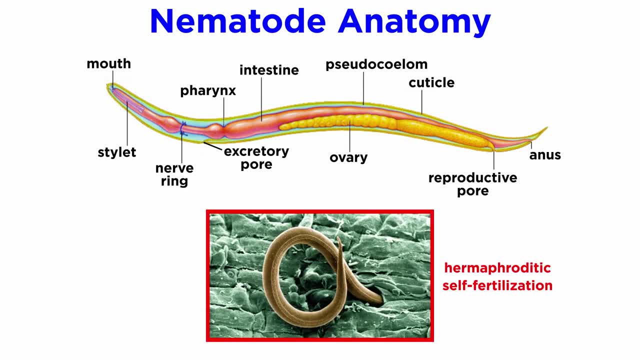 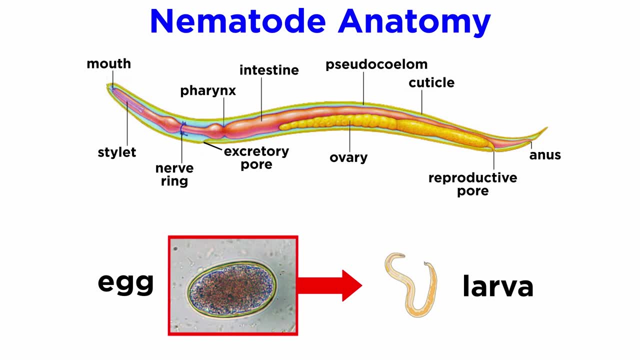 The fertilization process is internal and fertilized eggs are stored in the uterus. Though nematode reproduction is often sexual hermaphroditic, individuals are capable of self-fertilization. In most free-living nematodes, the eggs develop directly into larvae, which closely resemble. 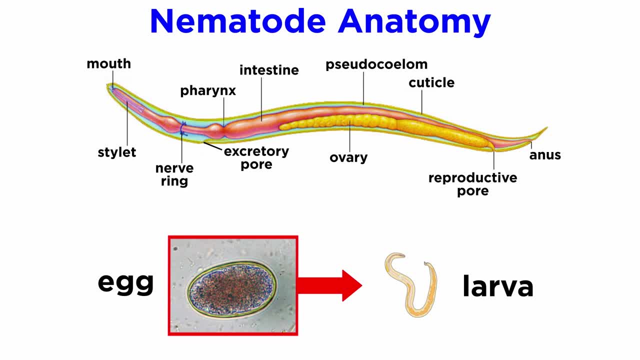 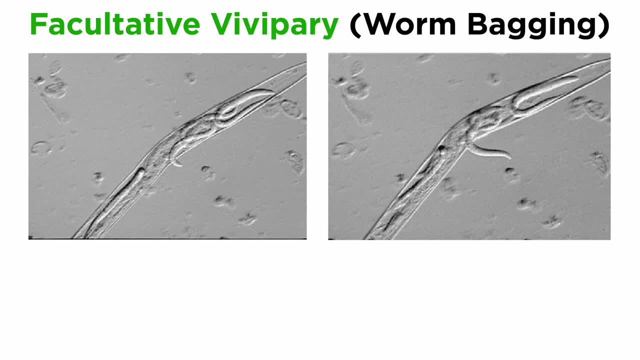 miniaturized versions of the parents, just with an underdeveloped reproductive system. Most species lay microscopic eggs that are protected by a tough outer shell, though some species, like C elegans, instead display a behavior known as worm-bagging or facultative. 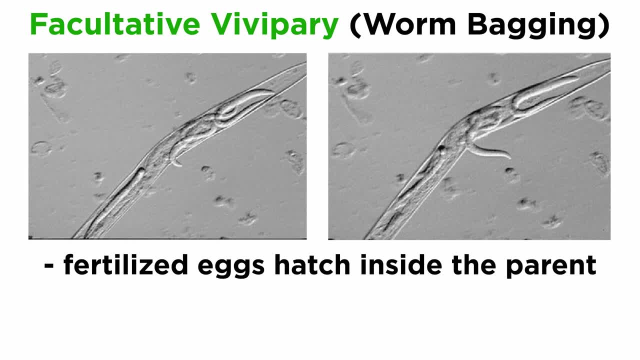 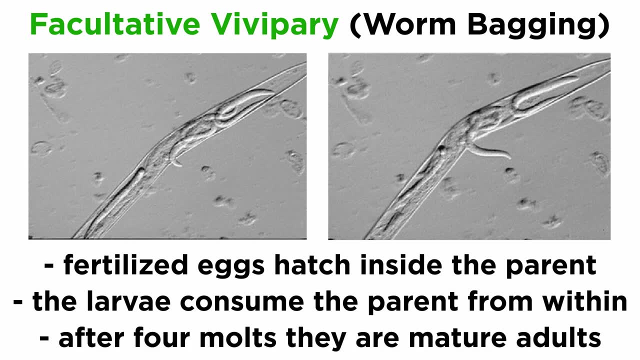 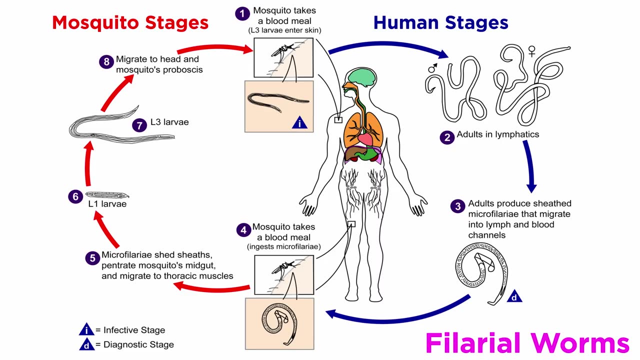 vivipary, where fertilized eggs hatch inside the parent and the larvae then consume their parent from within to emerge as juveniles. Regardless of how the juveniles hatch, After four molts of their outer cuticle they are sexually mature adults. 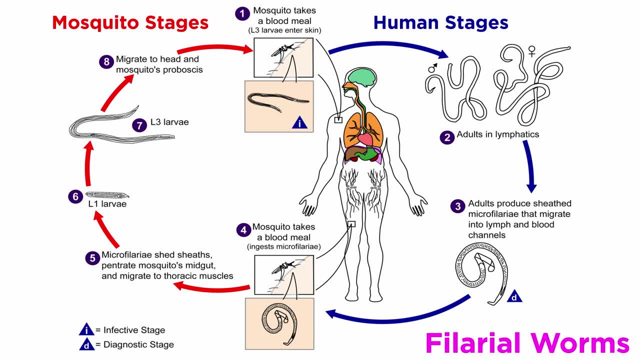 In parasitic species, reproduction is quite a bit more complicated and often involves several hosts, changes in morphology and a variety of different eggs. Falarial worms, for example, have different life stages in mosquitoes and humans and cycle between the two hosts to further infection. 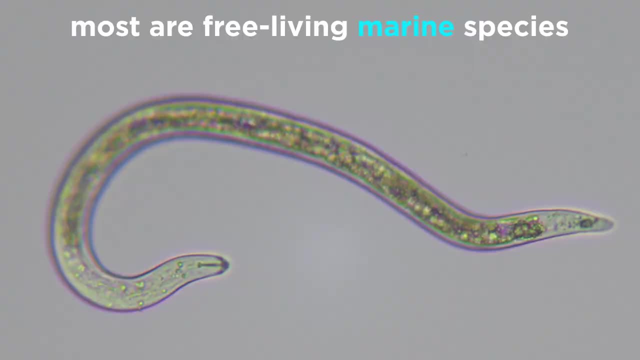 The majority of nematodes are free-living marine species, and a significant portion of them live in terrestrial or freshwater dwelling. By some estimates, they make up more than 90% of all species living on the ocean floor, though they are often ignored in favor of larger charismatic abyssal dwellers. 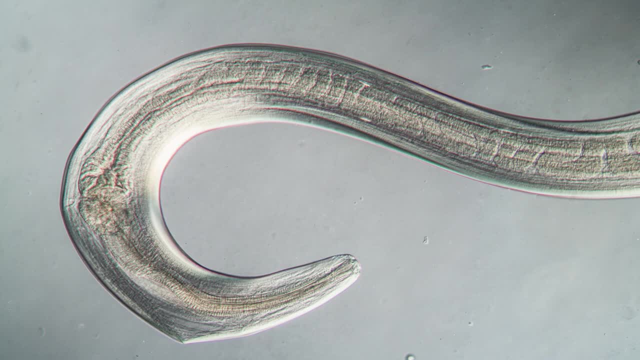 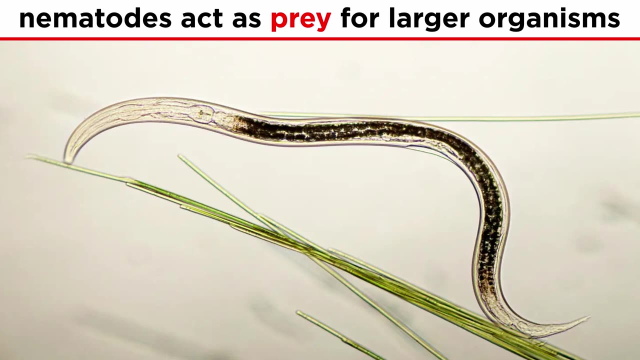 Their abundance and importance on our planet cannot be overstated. Some are herbivores, others are fungivores, bacterivores or predators. They provide an important ecological link, as a great deal of them are prey for larger soil-dwelling organisms. 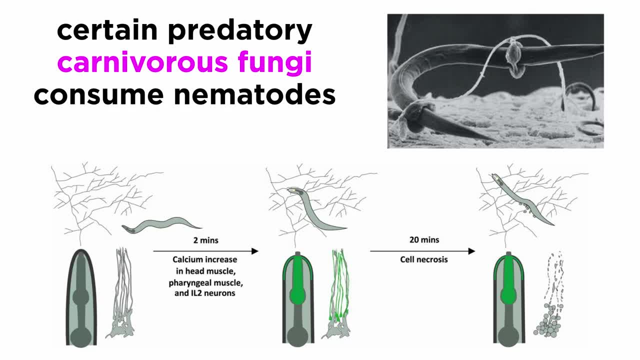 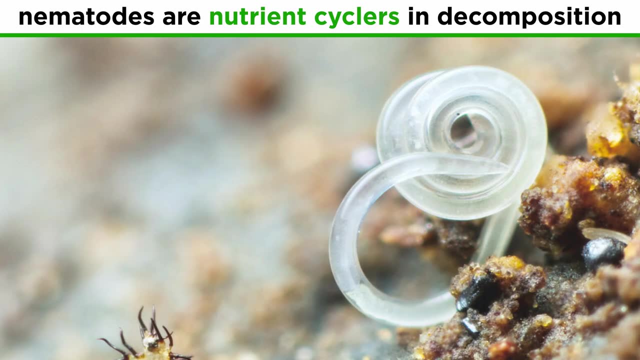 Some are even eaten by specially adapted predatory fungi that specialize in consuming nematodes. Some trap adult nematodes, others feed on eggs and still others produce toxins or invade the nematode Pseudocelum In the soil. nematodes are extremely important nutrient cyclers that play an essential role. 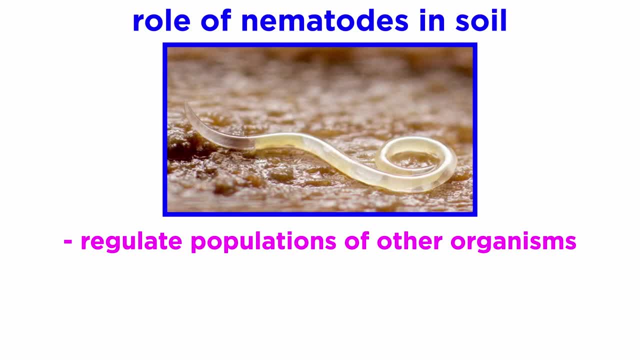 in the decomposition process. They regulate the populations of other soil organisms, mineralize nutrients in the soil and help the nematodes survive. They are also a great source of food for other organisms. They provide nutrients into plant-available forms, provide a food source for other soil. 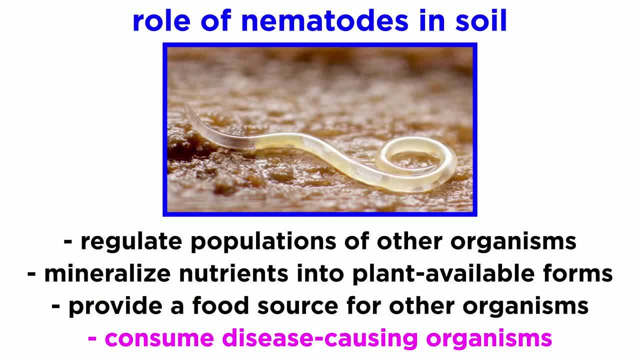 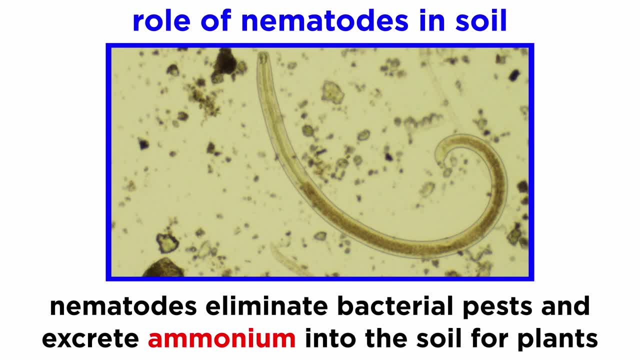 organisms and consume disease-causing organisms. For example, when a bacterium-feeding nematode consumes a disease-causing bacterium, the nematode not only eliminates the pest, but also excretes excess nitrogen in the form of ammonium, which is a plant-available form of nitrogen that aids in plant growth. 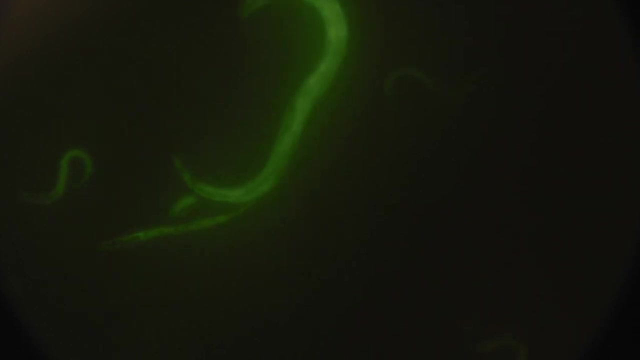 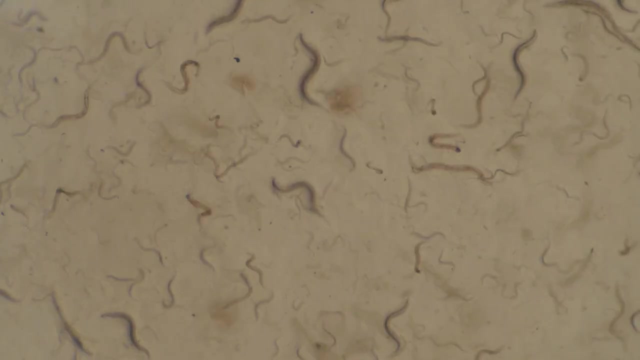 Other species of nematodes play similar but different roles. They play distinct roles in freshwater and marine systems, where they are especially important in the decomposition process, But others also cycle nutrients, feed on algae and microscopic diatoms, stimulate nutrient remineralization and also serve as indicators of biological health, since some species are 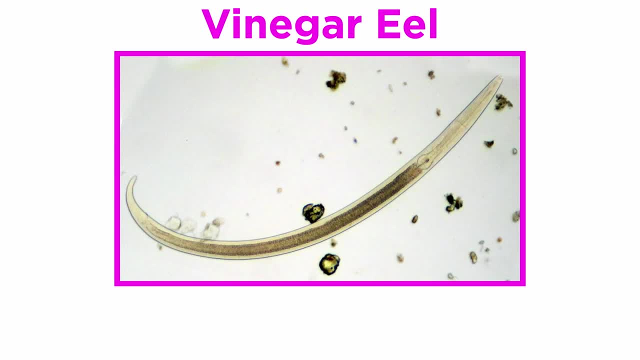 very sensitive to pollution. Other species of nematodes live in our food, like the vinegar eel that was first discovered in unfiltered vinegar. It has been found to survive in a pH range of less than 1.6, which is lower than stomach. 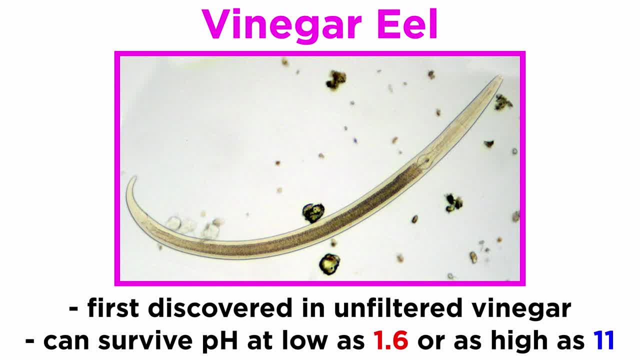 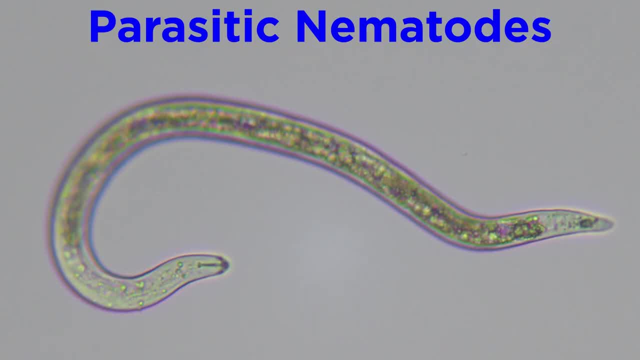 acid or pure lemon juice and up to 11, about as basic as ammonia. Thankfully, they are harmless, non-parasitic and filtered out of most vinegar. Unfortunately, not all species of nematodes are free-living. Some species of nematodes are significant agricultural pests that can parasitize crops. 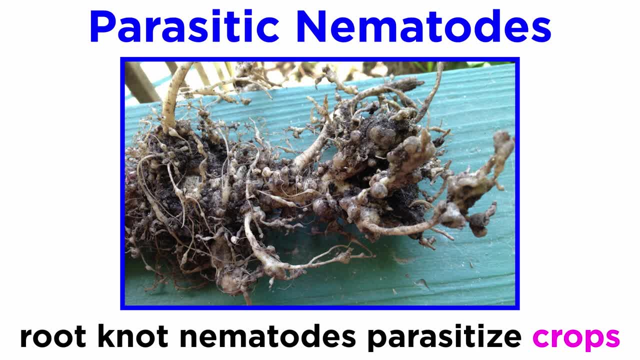 and cause significant damage. The root knot nematodes, for example, are a very common species of nematodes. They are a very common species of nematodes. They are a very common species of nematodes. They are often considered some of the most damaging pests to household gardens. 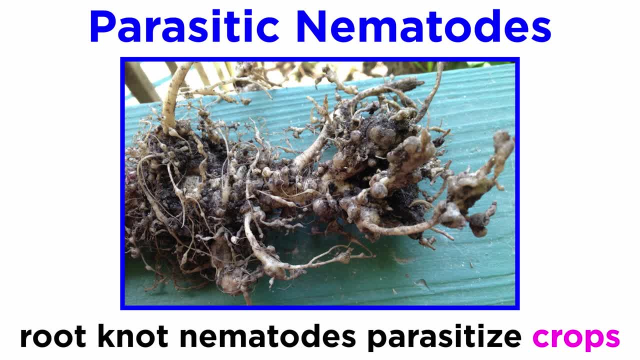 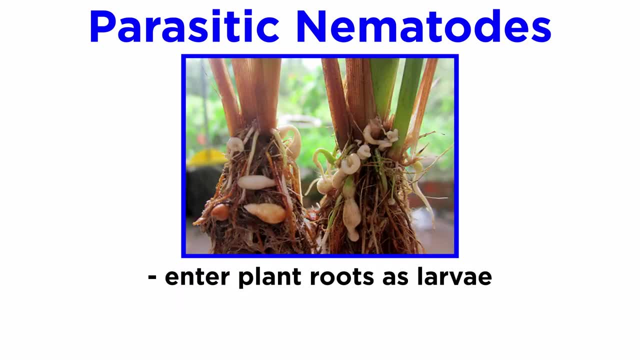 Unlike most pests, they are generalists rather than specialists and can parasitize more than 2,000 plant species. They enter plant roots as larvae, mature and mate within the roots and lay eggs in the surrounding soil. The galls or knots damage the plants by blocking the flow of water and nutrients and allowing 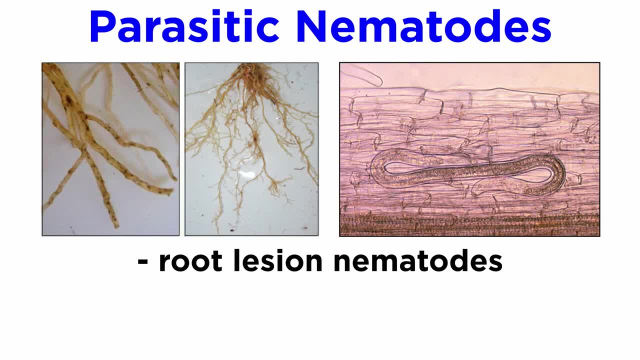 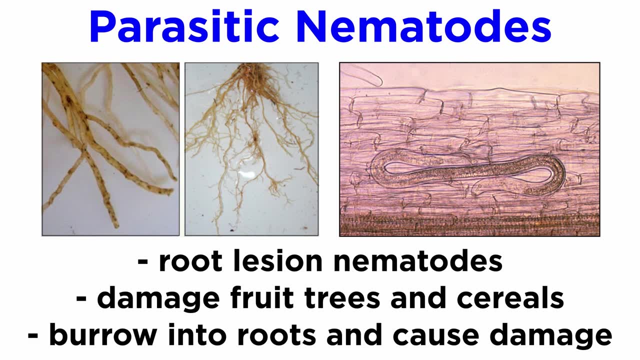 pathogens to invade. The most common nematode pests are root lesion nematodes, which damage fruit trees and broad acre crops like cereals. There they burrow into roots and extract cell nutrients, damaging feeder roots and causing the plant to create a weak shallow root system with many dead or drying areas. 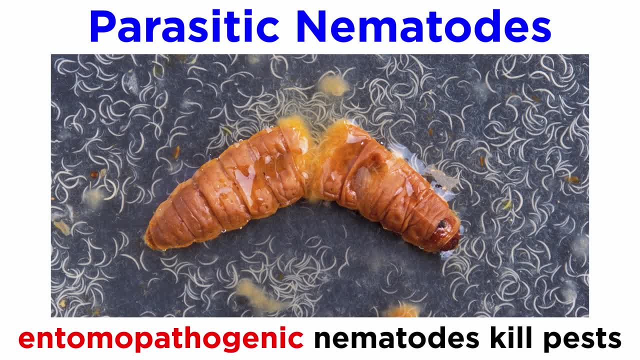 However, not all nematodes negatively impact crops. In addition to the thousands of species of harmless soil-dwelling nematodes, there are also entomopathies. Entomopathies are entomopathogenic species which selectively parasitize insects. 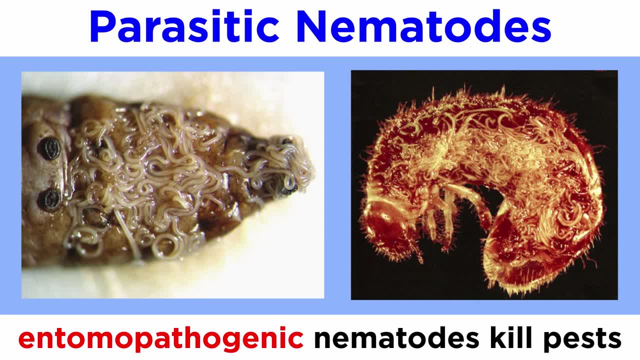 Some infect larval forms and others infect adults. They have been found all over the world and are highly diverse, complex and specialized. They have been used as a form of biological control and spread by farmers through crops infested with specific insects. 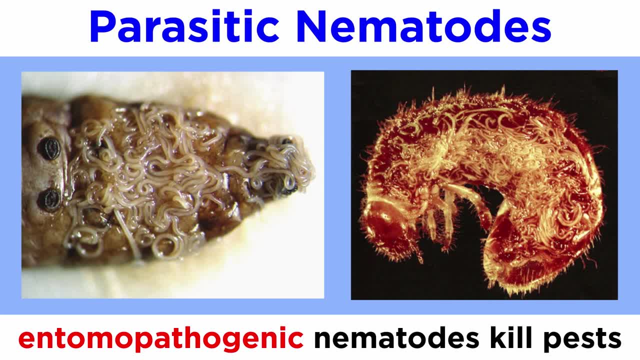 They act kind of like a living pesticide and they don't leave any chemical traces. Since they are microscopic, they can be applied to crops using a variety of pesticides. They can be applied to crops using a variety of pesticides. They can be applied to crops using a variety of pesticides. 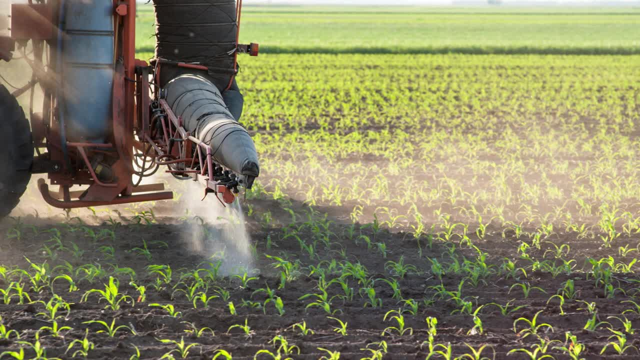 Kind-of. both of these soortes are sprayed with a variety of pressurized sprayers alongside or instead of traditional pesticides and fertilizers. However, although they have been used since the 1980s, there is a lack of fundamental research on the potential for their widespread use. 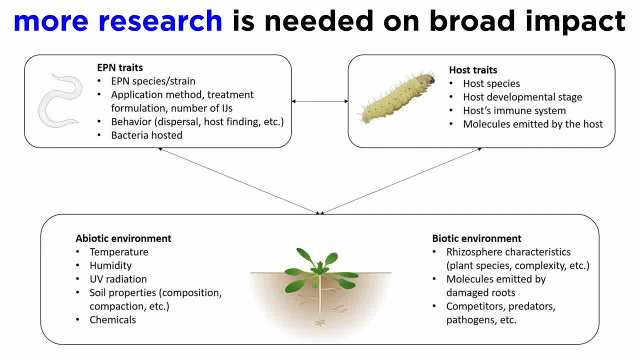 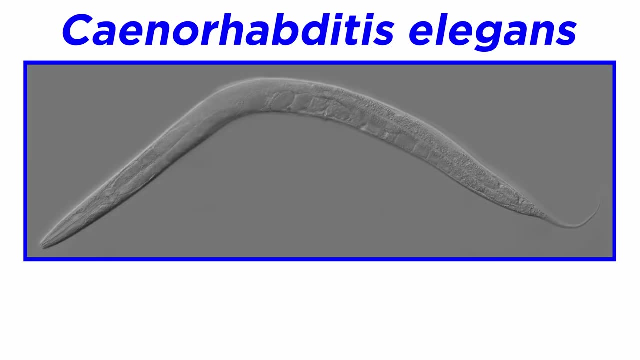 Though they can easily be mass-produced and selectively target pest species, there are still some concerns about their long-term continued use in agriculture. However, they could serve as non-toxic alternatives to some current pesticides. Thanks teams, Thanks Whiteoken. The last species of nematode we will mention here is C elegans, perhaps the most scientifically. 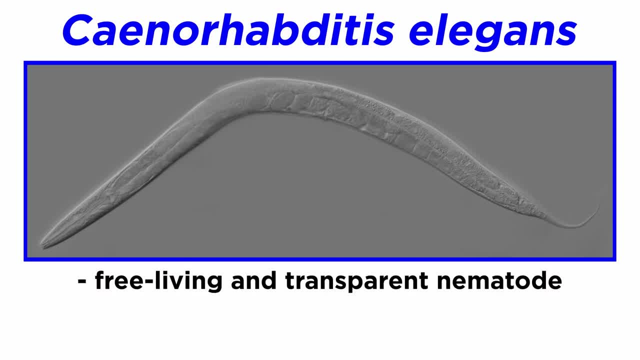 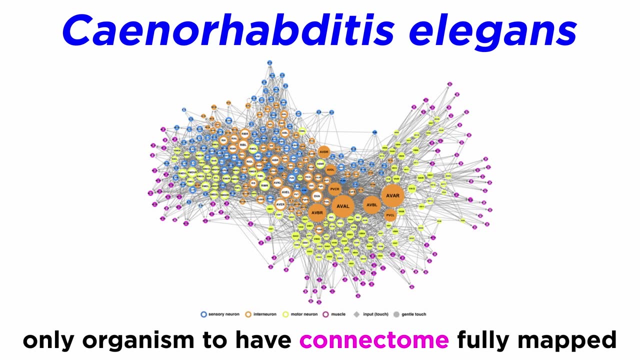 significant species of nematode. C elegans is a free-living transparent nematode about one millimeter in length that is common in temperate soil environments. It was the first multicellular organism to have its entire genome completely mapped and it is currently the only organism to have its connectome completed, which is a map of. 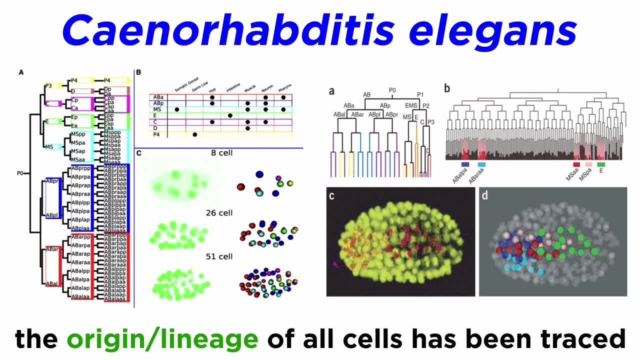 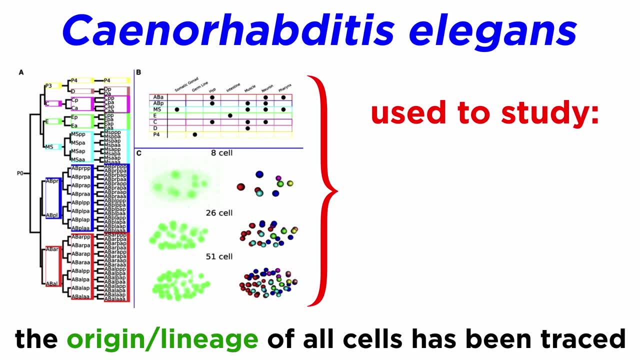 brain connections. The origin and lineage of all the cells of its body have been traced from zygote to adult, and it has been used as a model organism in studies regarding cell lineage mapping, programmed cell death, RNA interference and gene silencing, cell division and the cell cycle, drug abuse.